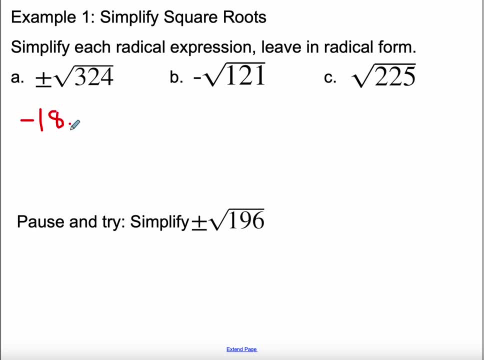 And positive 18, because it's asking for both positive and negative. because of this plus or minus symbol, For the middle one we have the negative square root of 121.. So, because it's asking for the negative one, I just need a negative answer. So, if I do the square root, 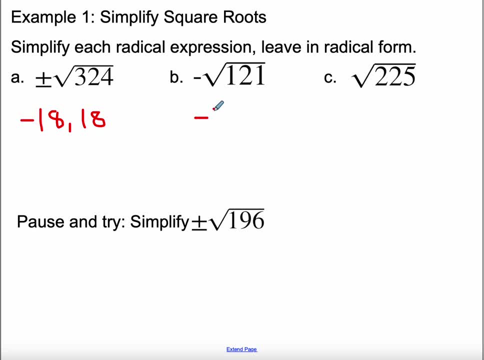 of 121, my calculator says that it is 11.. So my answer for B would be negative 11.. And when I do the square root of 225, the square root of 225 is 15.. Now this one isn't asking. 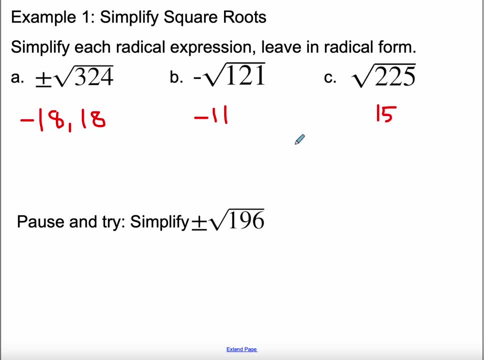 specifically for either positive or negative, And so most of the time we can assume that it's asking for a positive answer. So at this time, pause and simplify the plus or minus square root of 196.. So the answer? what do you? 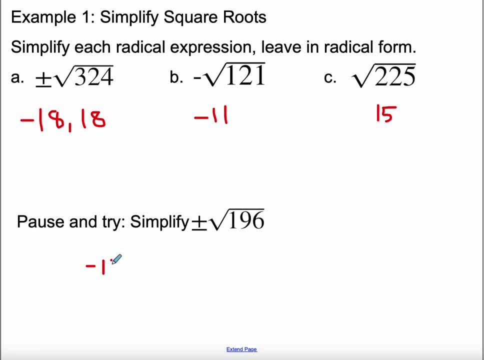 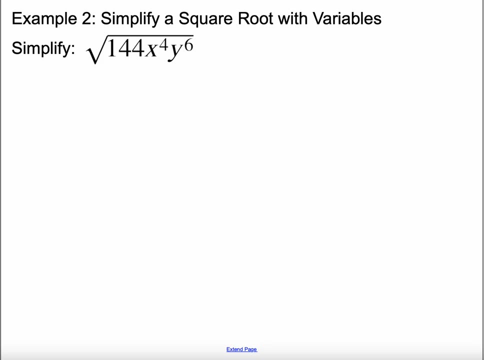 what do you think about this? That's a really good question And if you think about it, that is the answer. You can't really make an answer out of a zero, So I'm gonna read through it And the answer to this is: the answer to this is negative 14 and positive 14.. Now, when I add in variables underneath the radical, it's not much difference, And so one of the things that I know that a variable is a perfect square is by whether or not the exponent is an even number. So when I'm dealing with square roots, I'm gonna say: 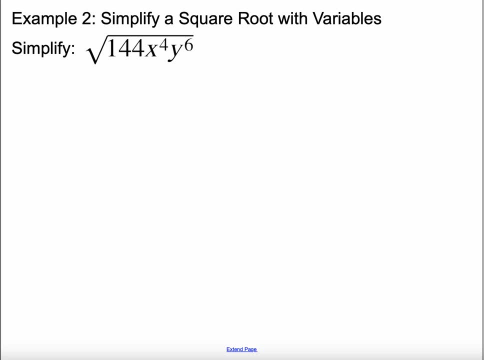 I'm gonna say I'm looking for an even number for exponents, And so the square root of 144 is 12.. Now for this x to the 4, it's actually pretty simple to find the square root of x to the 4th. 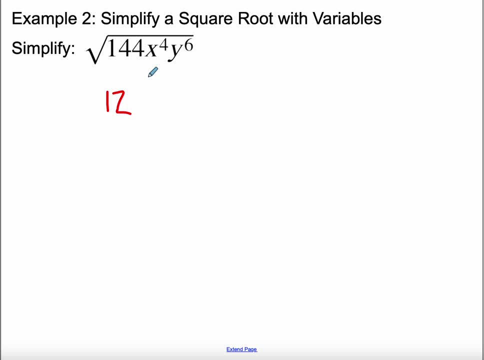 Because we're going to take our exponent of 4 and divide it by 2.. And so the square root of x to the 4th is x squared. Same thing with y to the 6th. I'm going to take my 6th and I'm going to divide it by 2.. 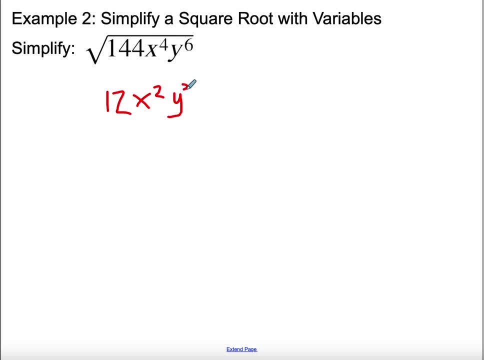 So the square root of y to the 6th would be y to the 3rd, And so my final answer for this problem is: 12x squared y to the 3rd.